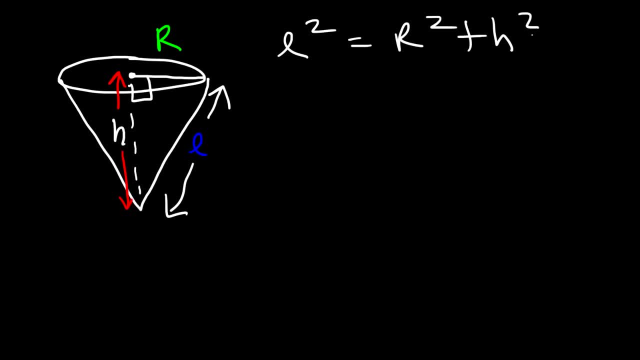 C squared is A squared plus B squared. So that's the equation. you need to relate R, H and L together. Now, in order to find the volume of a cone, you need to use this equation. It's one-third base times height, where B represents the base of. 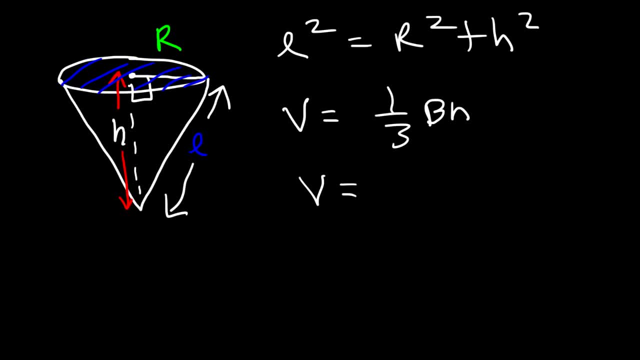 B is the area of the base, which is basically the area of the circle, So it's one-third pi R squared times height. The area of a circle is pi R squared, So combined this gives you the volume equation of a cone. 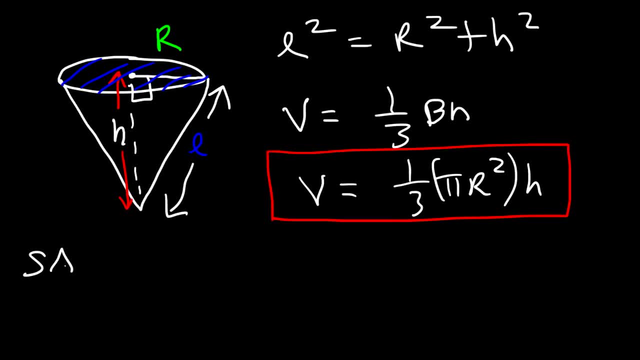 Now, in order to find the surface area, you need to know that the surface area is the area of the base plus the lateral area. The lateral area is pi times R times the slant height L. The area of the base is pi R squared plus the lateral area, which is pi R L. 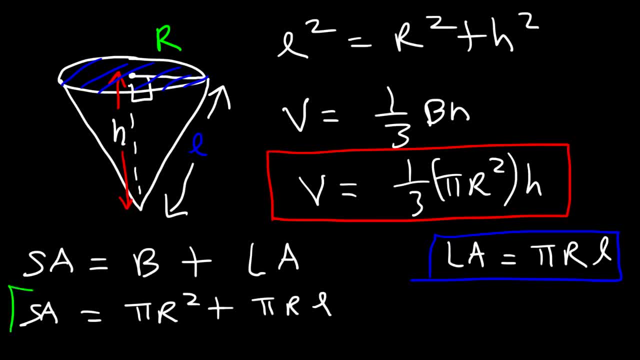 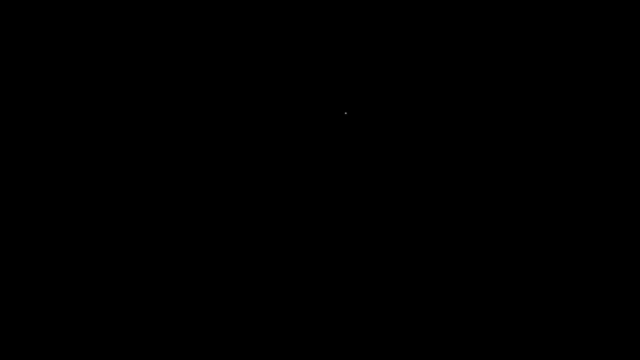 So combined, this will give you the surface area. So these are the equations That you need to find: the volume of a cone, the lateral area and the surface area. So let's work on an example. Let's say the radius of a cone is 5 centimeters. 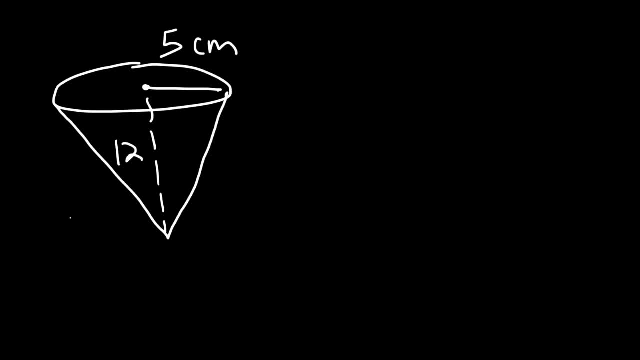 And the height of the cone is 12 centimeters. Using this information, go ahead and find the volume, the lateral area and the surface area. So let's start with the volume. We know the volume is one-third the area of the base, which is pi R squared times the height of the cone. 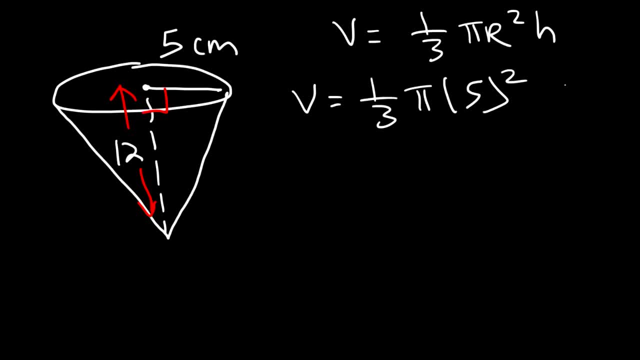 So we have the radius, which is 5, and the height is 12.. 5 squared is 25.. And 25 times 12.. If you have 12 quarters, that would be $3.. $3.. $3.. 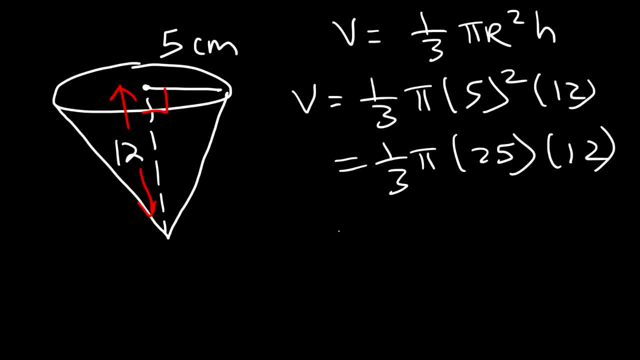 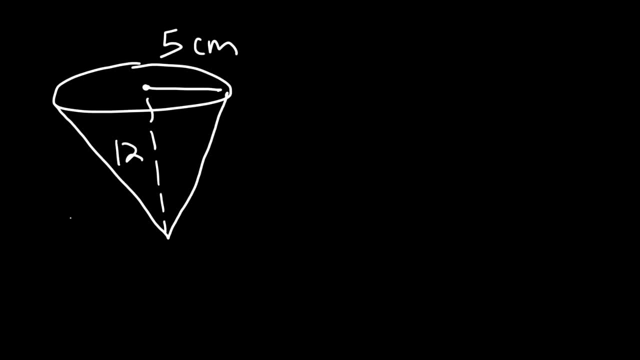 And the height of the cone is 12 centimeters. Using this information, go ahead and find the volume, the lateral area and the surface area. So let's start with the volume. We know the volume is one-third the area of the base, which is pi R squared times the height of the cone. 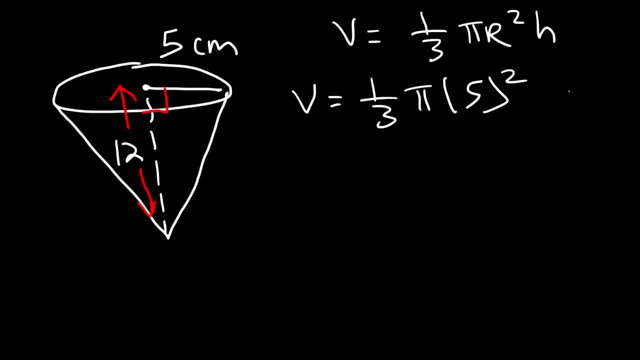 So we have the radius, which is 5, and the height is 12.. 5 squared is 25.. And 25 times 12.. If you have 12 quarters, that would be $3.. 25 times 12 is 300.. 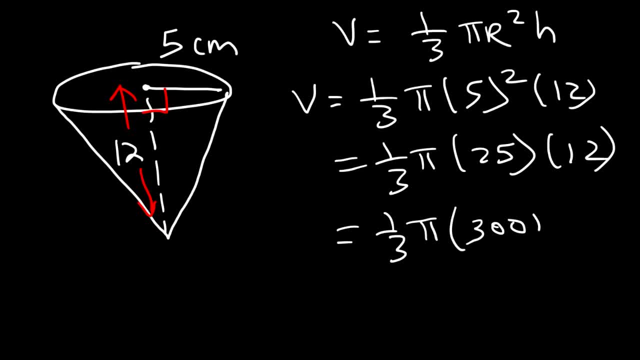 So this is one-third pi times 300, and one-third of 300 is 100.. So the volume is 100 pi And the units is going to be cubic centimeters. Now how can we find the lateral area? 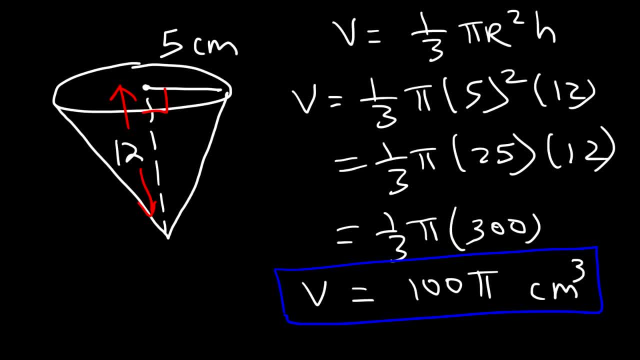 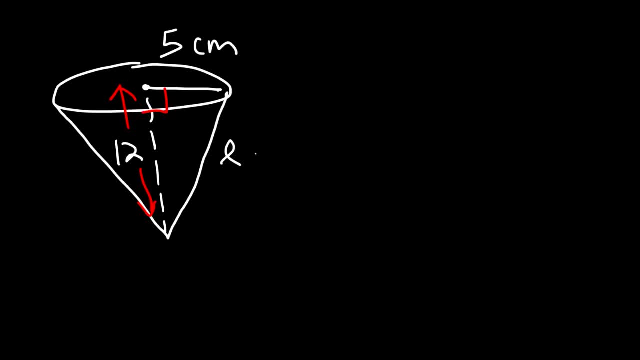 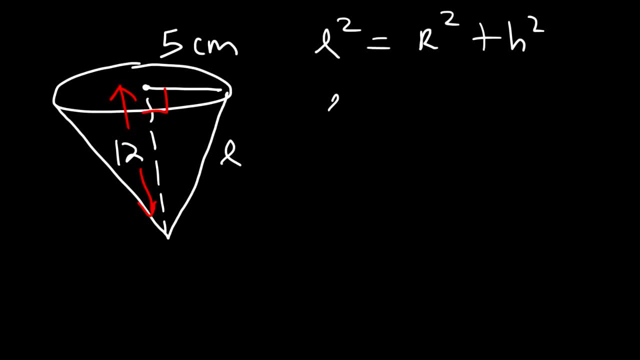 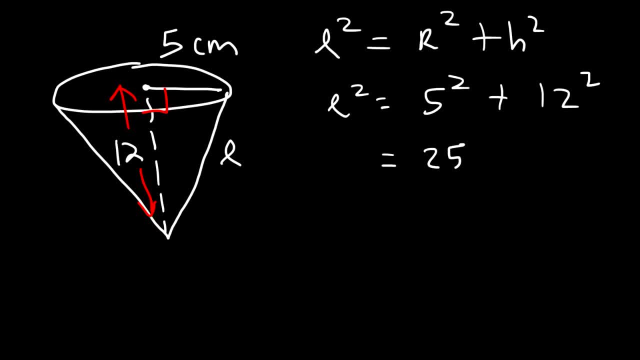 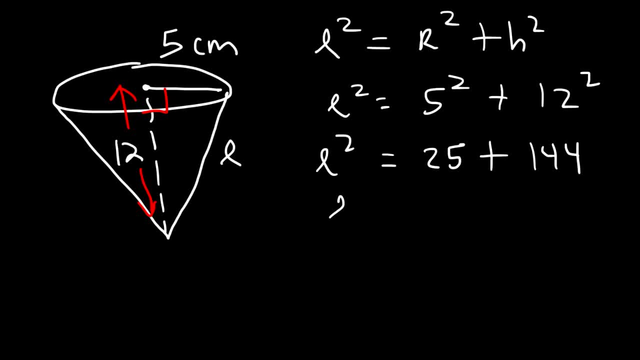 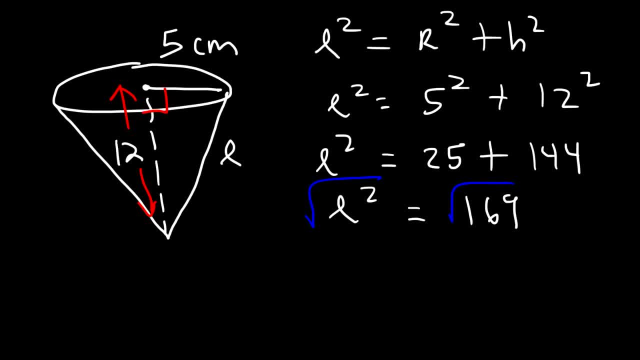 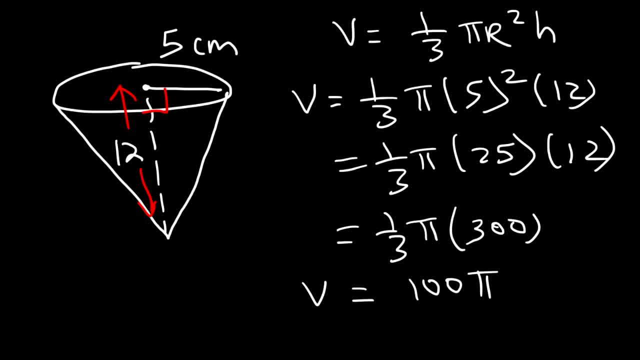 So the volume is 100 pi And the units is going to be cubic centimeters. Now how can we find the lateral area? Feel free to pause the video and go ahead and find the lateral area. Before we could find the lateral area, we had to find the surface area. 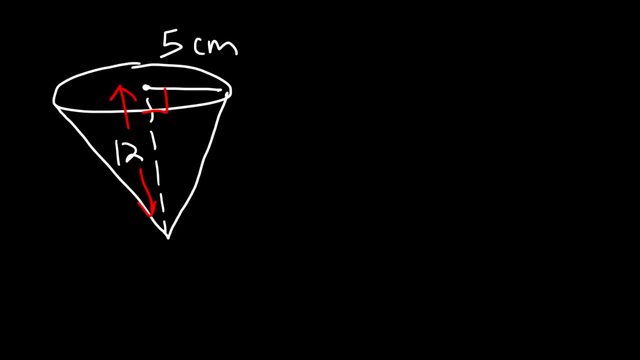 Before we could find the lateral area, we had to find the square area And we need to calculate the slant height. So we have to find L. Let's use this equation first: L squared is equal to R squared plush squared. 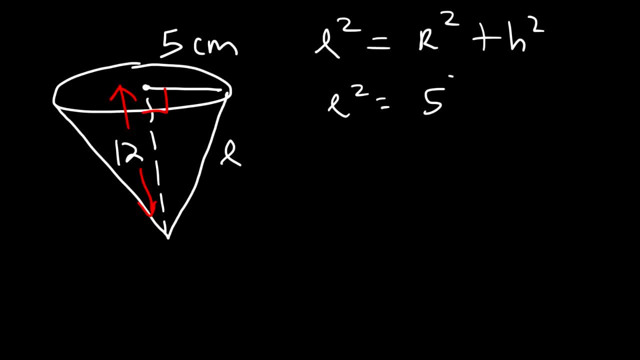 So R is 5.. h is 12.. 5 squared, or 5 times 5, that's 25.. 12 squared, 12 times 12 is 144.. And if we add those two numbers, that's going to give us 169.. 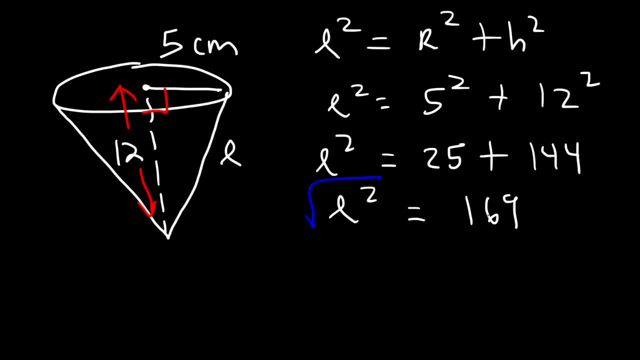 And then we have to find the slant height. So we have to find the slant height, So we have to find the slant height. Now let's take the square root of both sides. The square root of L squared is L. 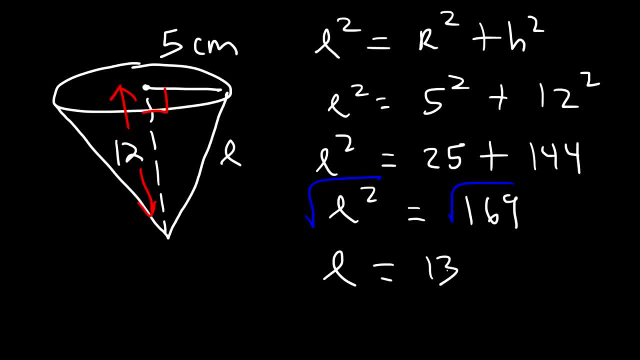 The square root of 169 is 13.. So L is 13 centimeters long. So now that we have the value of L, we can find the lateral area. It's pi times R times L, So that's pi times 5 centimeters times 13 centimeters. 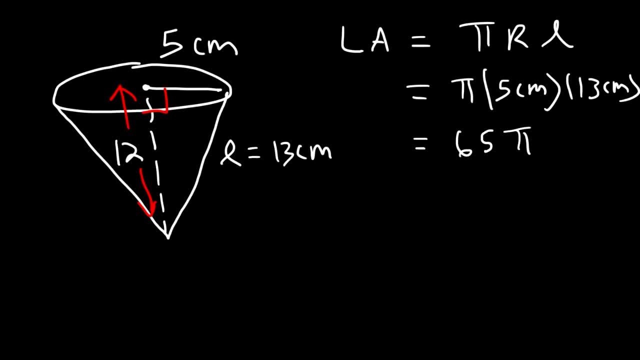 5 times 13 is 65.. Now what are the units for lateral area? Well, if you multiply centimeters by centimeters, you're going to get square centimeters. So anytime you're dealing with area, it's going to be square units. 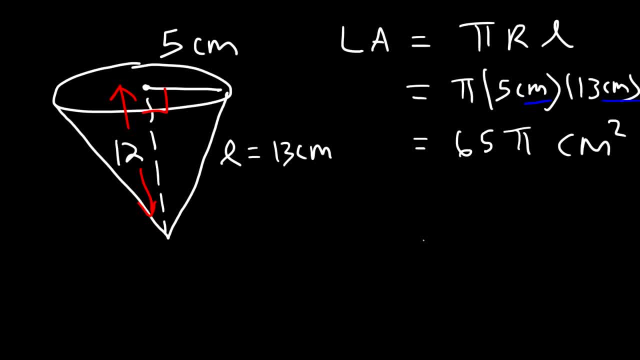 With volume cubic units or units cubed. So the lateral area is just 65 pi square centimeters. So now that we have the lateral area we can find the surface area. The surface area is the area of the base plus the lateral area. 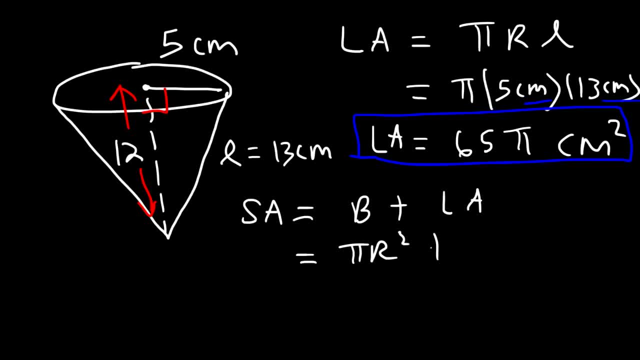 So the area of the base is pi R squared. The lateral area is pi R L. So this is going to be pi times 5 squared, plus pi times 5 times 13.. So that's pi times 5 squared. 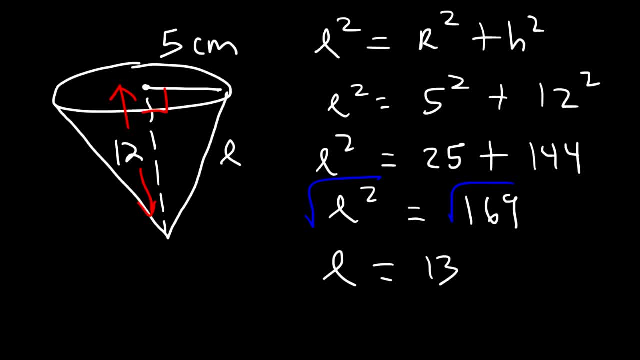 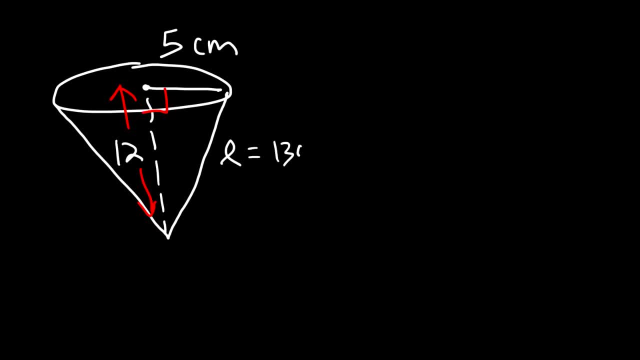 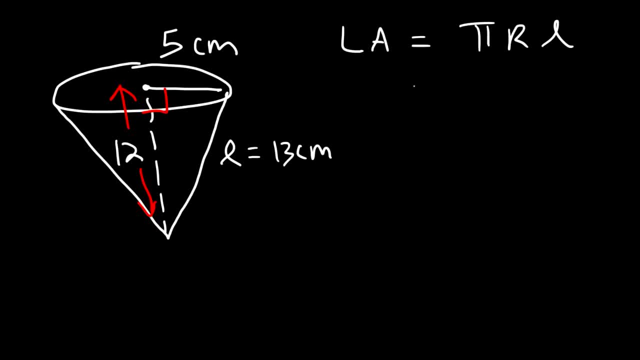 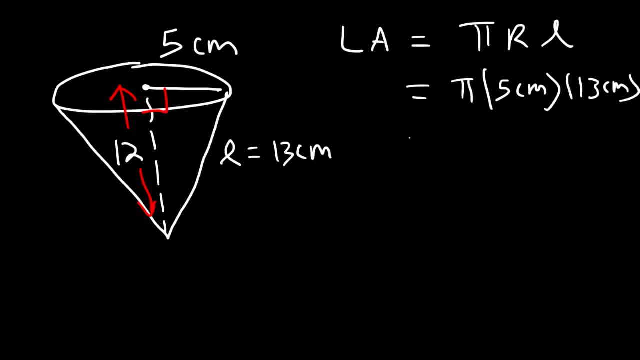 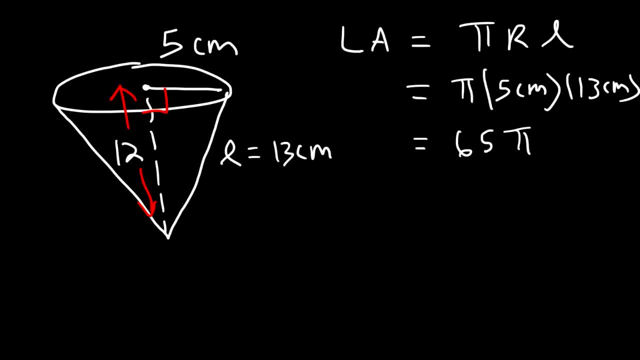 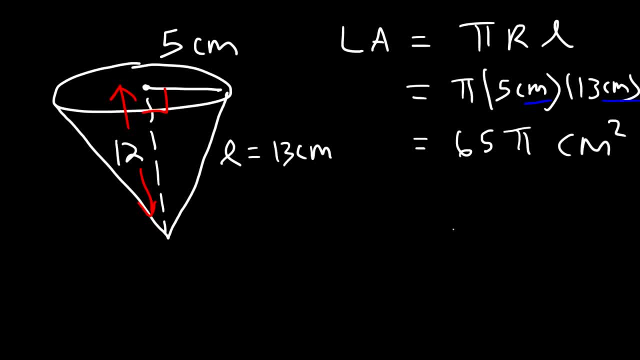 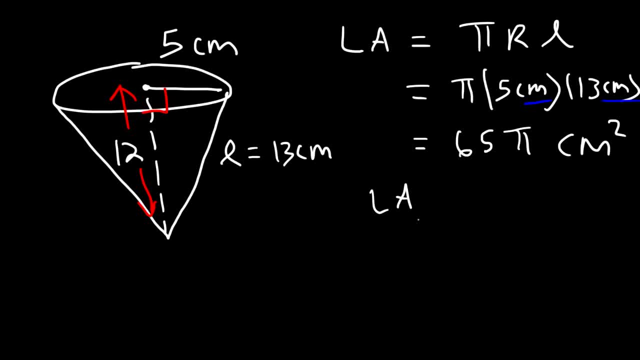 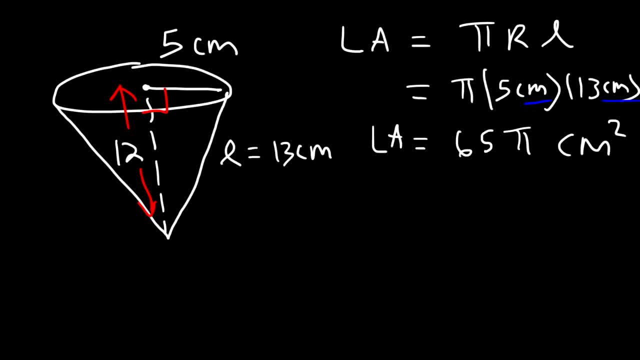 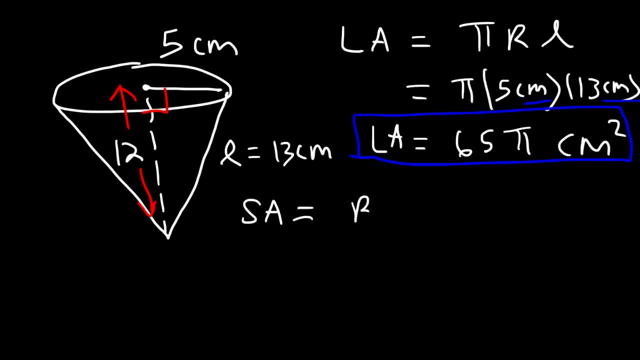 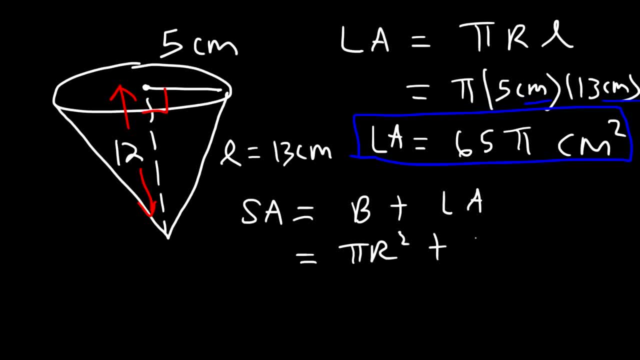 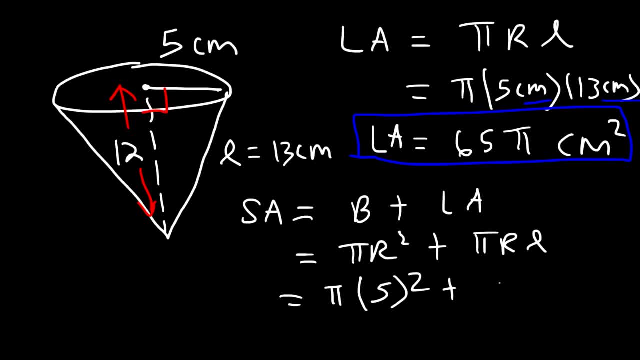 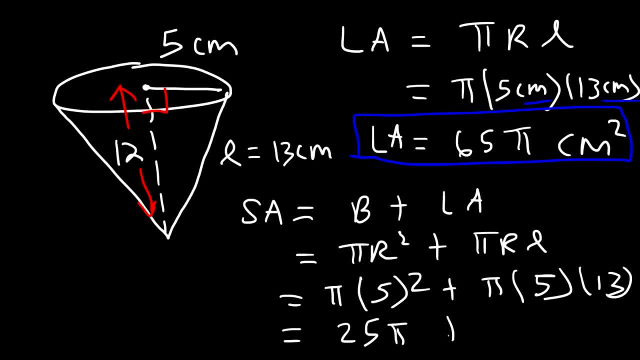 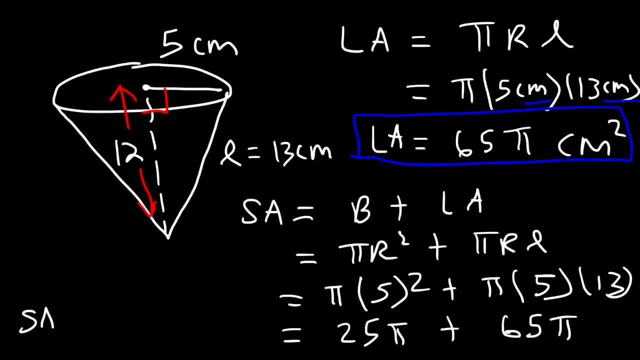 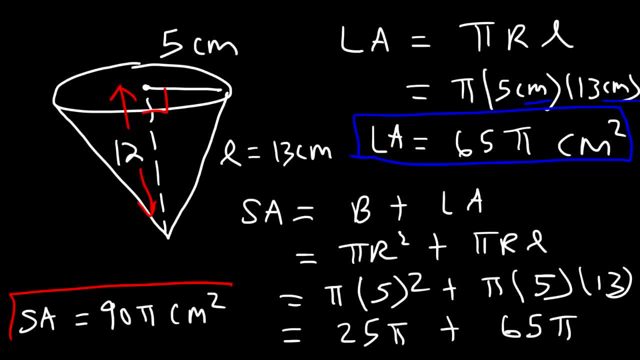 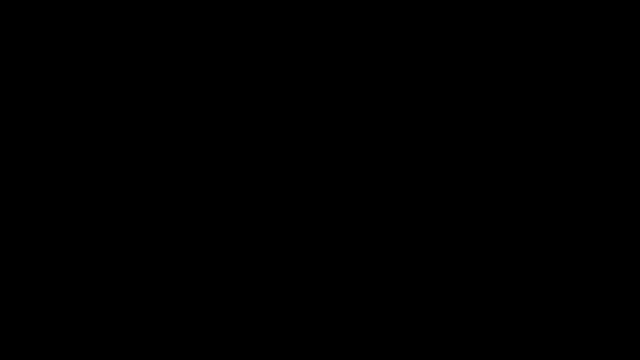 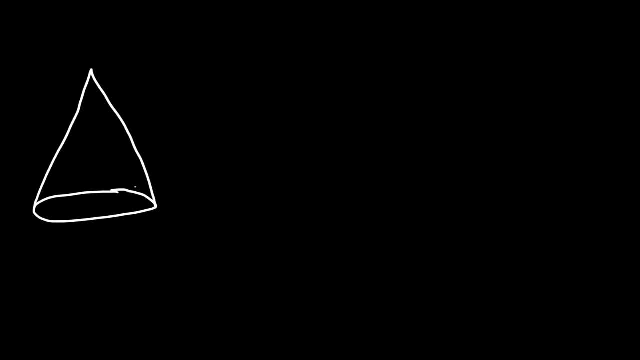 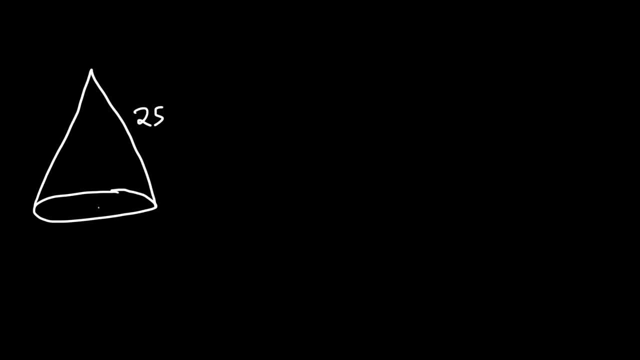 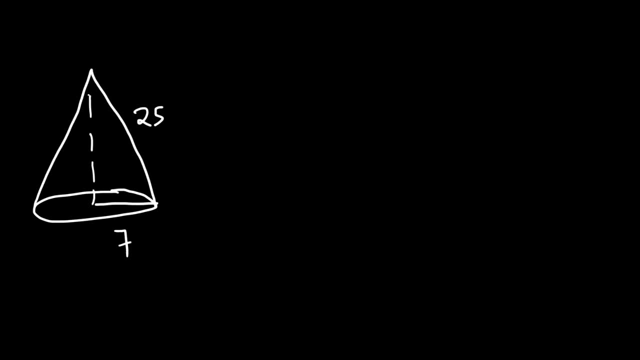 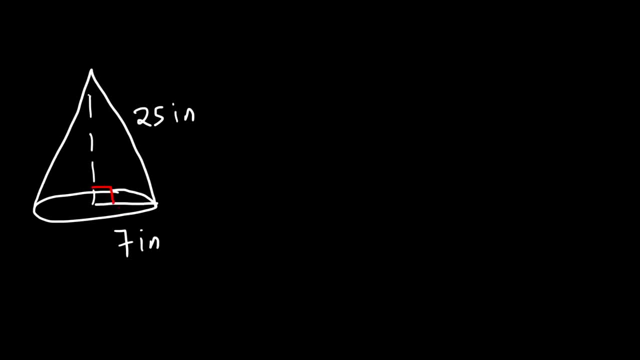 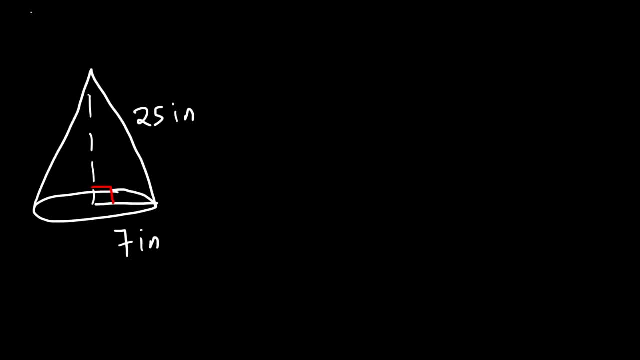 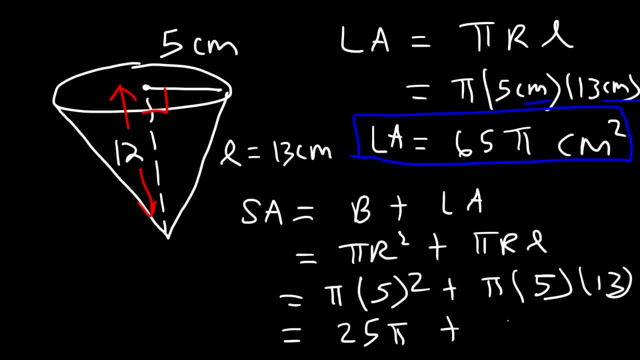 So 5 squared is 25.. And we know, 5 times 13 is 65.. 25 plus 65,, that's 90. So the surface area is 90 pi squared centimeters. So now you know how to find the volume, the lateral area and the surface area of a cone. 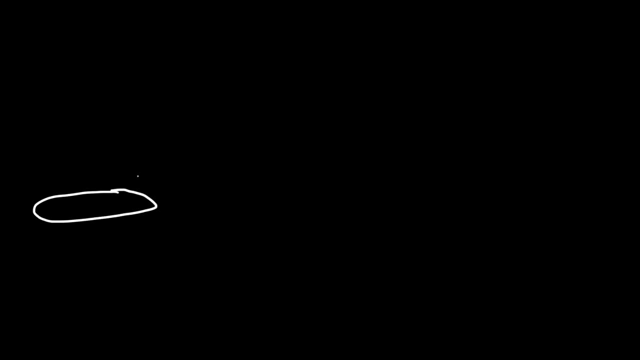 Let's work on another example. So this time let's say we're given the slant height and the radius. Let's say the radius is 7 inches and the slant height is 25 inches. So feel free to pause the video. 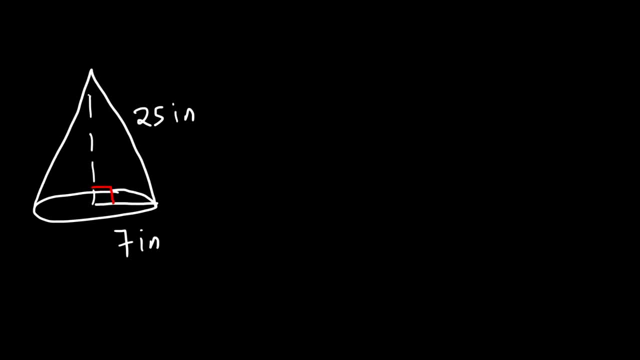 Go ahead and calculate the volume, the surface area and the lateral area. So we know that R is 7. And L is 25. What we need to find is H, So let's use the Pythagorean Theorem to calculate it. 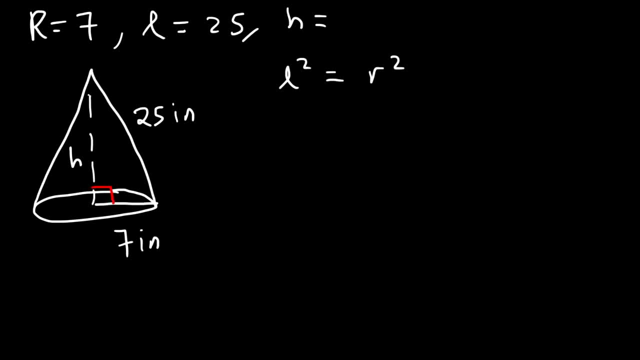 So we know that L squared is equal to R squared plus H squared. So L is 25.. R is 7.. And let's find the value of H. 25 squared is 625.. 7 squared is 49.. 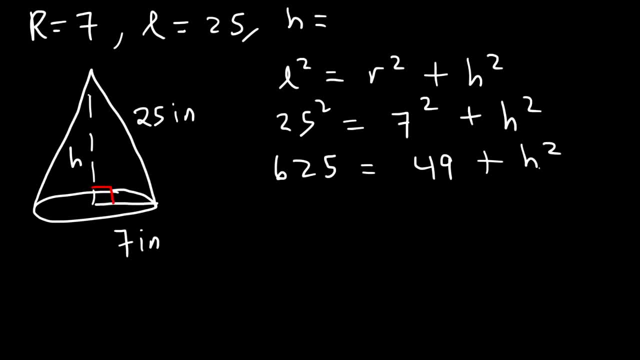 Now, in order to get H squared, we need to find the value of H by itself. we have to subtract both sides by 49.. So 625 minus 49, that's going to be 576.. So that's equal to H squared. 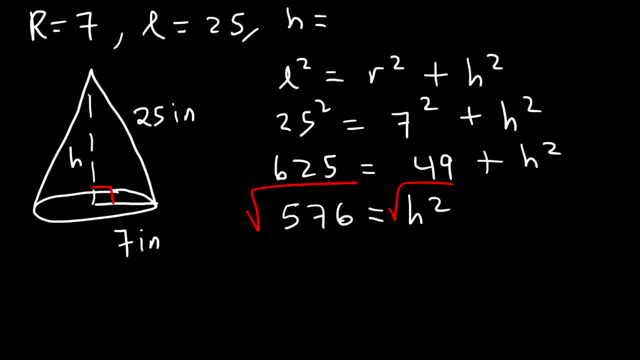 Now our next step is to take the square root of both sides And the square root of 576, that's going to give you 24.. So that's the value of H. H is 24 inches. Now that we have the value of H, let's go ahead and calculate. okay, what just happened. 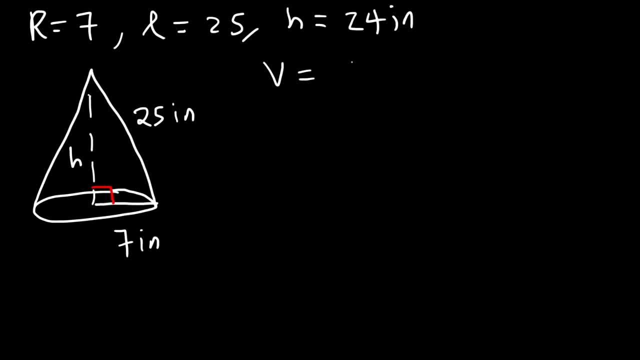 Let's go ahead and calculate the volume. So the volume is going to be 1 third pi R squared times H. So R in our example is 7 and H is 24.. Seven squared So, 7 times 7, that's 49.. 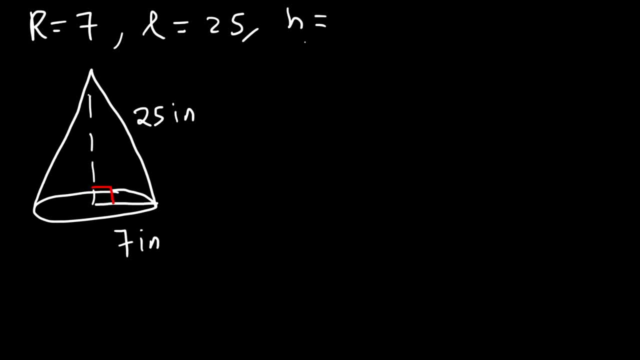 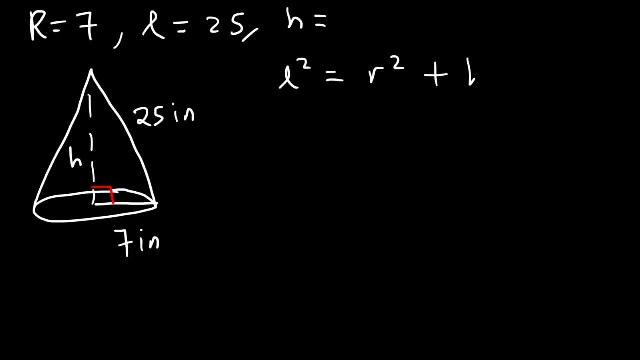 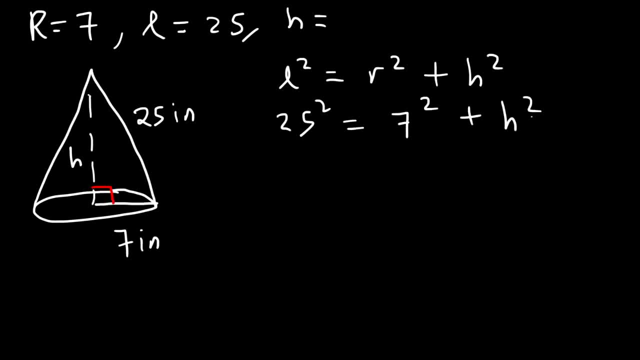 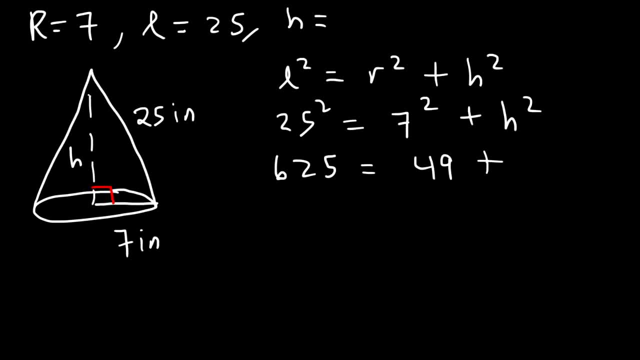 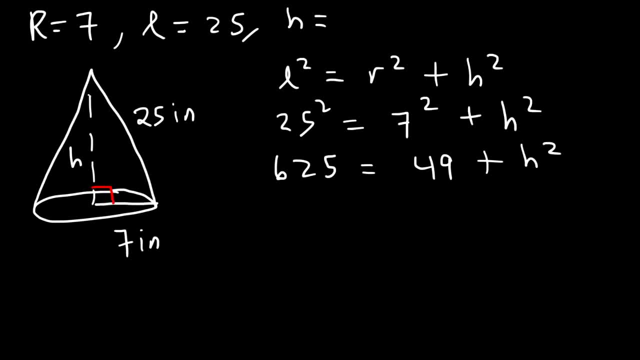 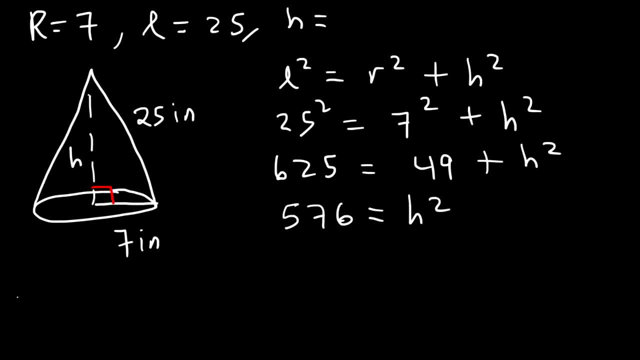 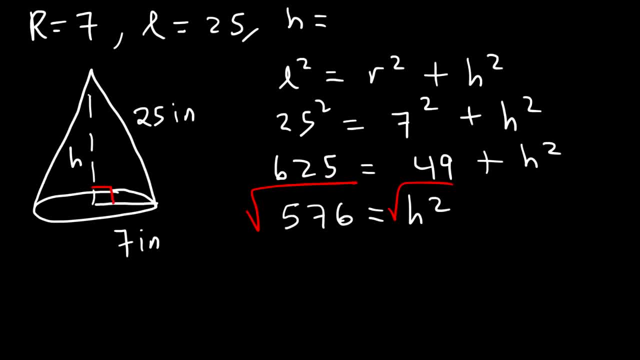 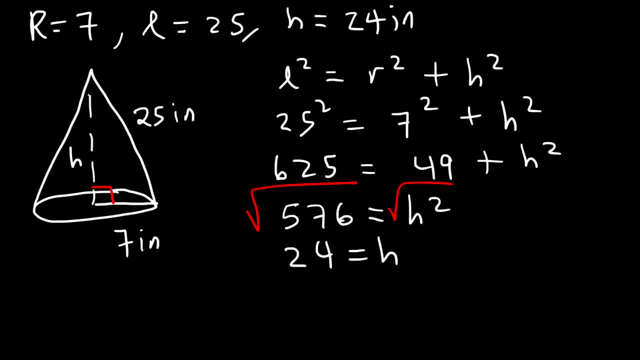 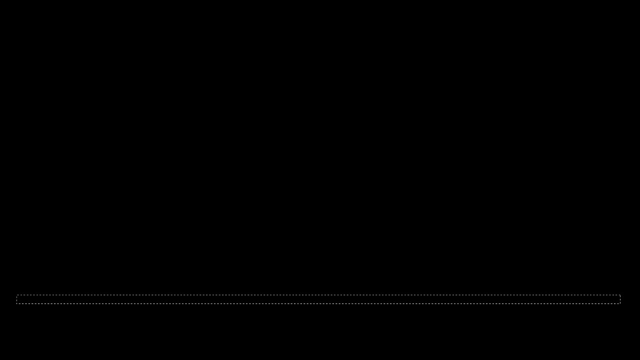 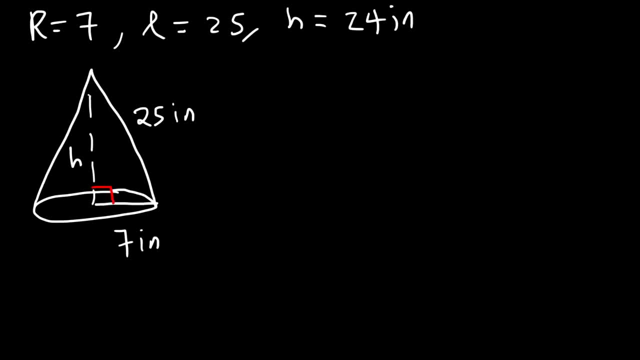 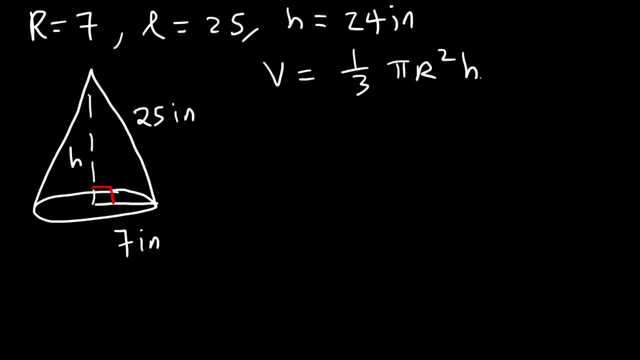 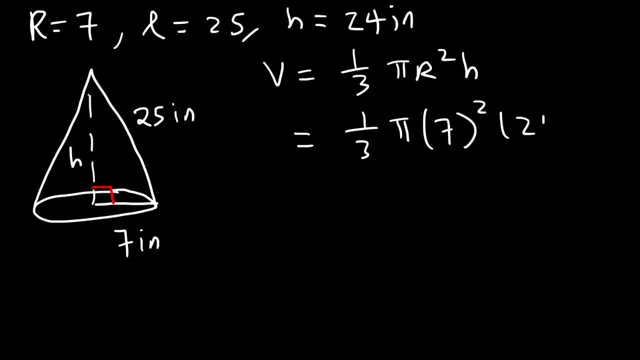 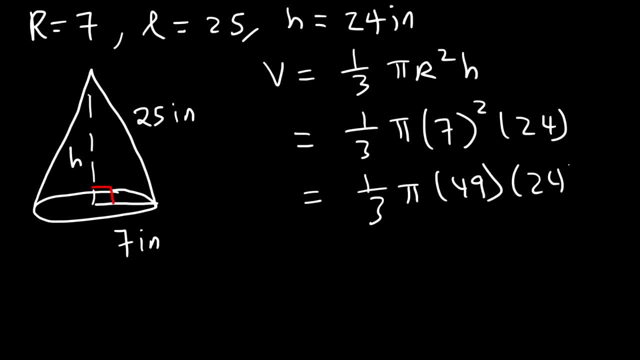 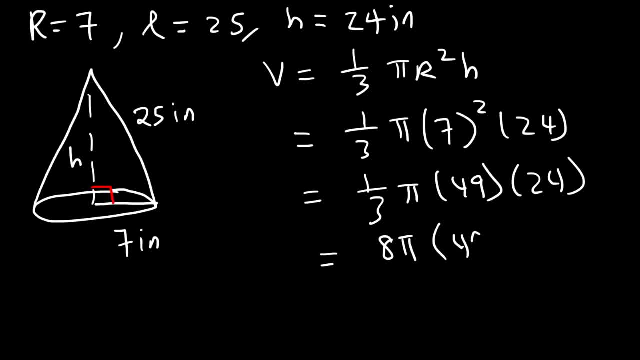 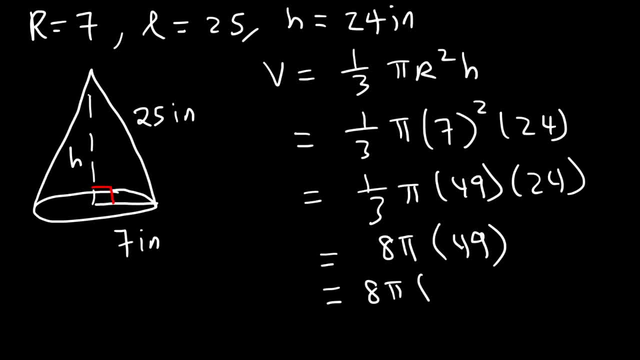 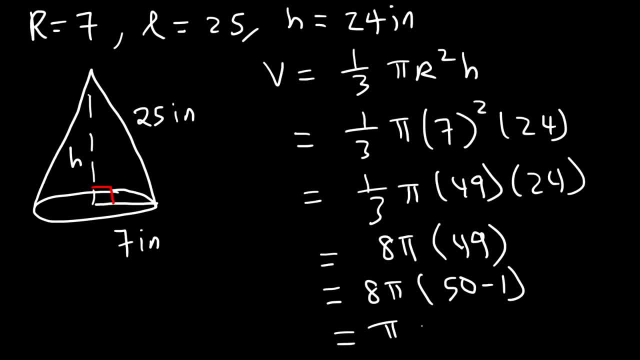 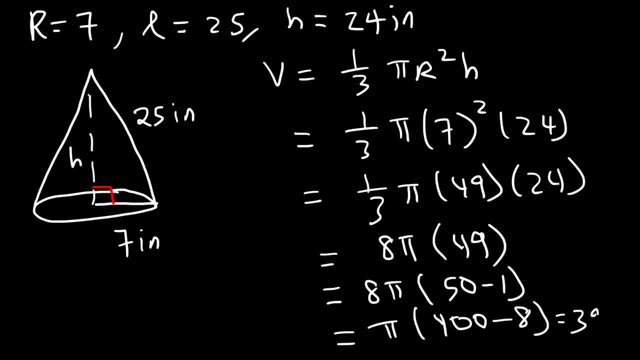 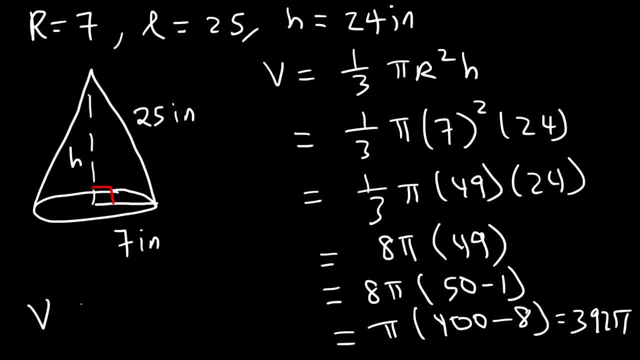 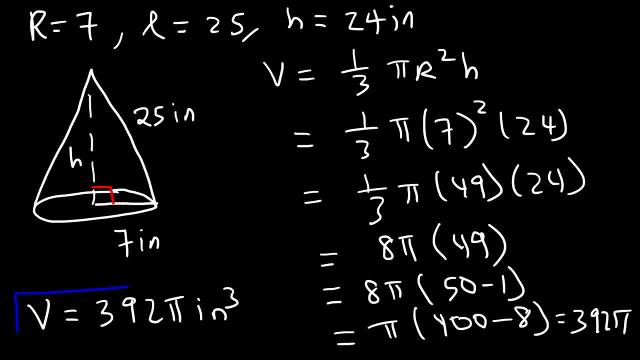 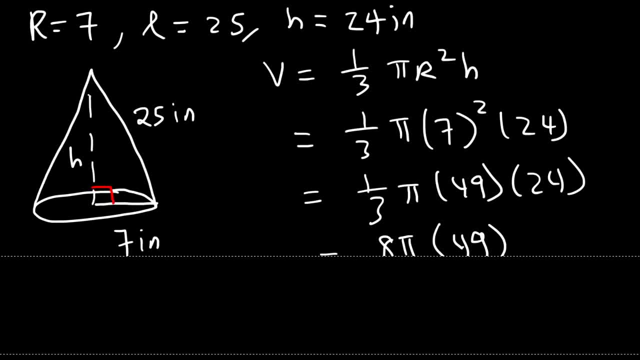 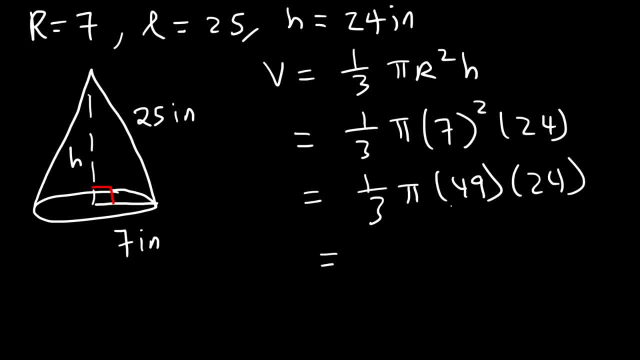 One third of 24, if you do 24 divided by 3, that's 8.. So we have 8 pi times 49.. When multiplying 8 times 49, if you want to do it in your head, replace 49 with 50 minus. 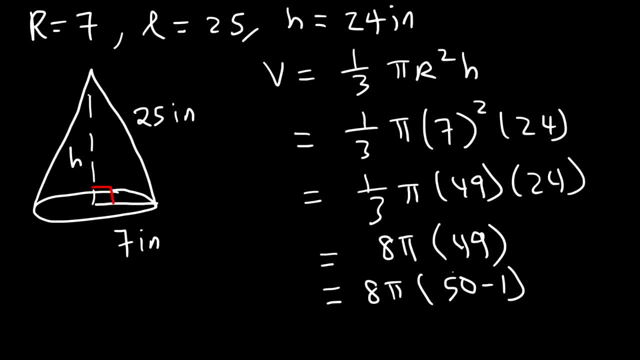 1.. 8 times 5 is 40. So 8 times 50, that's going to be 400.. And 8 times 1 is 8.. So if you subtract 400 by 8. You get 392.. 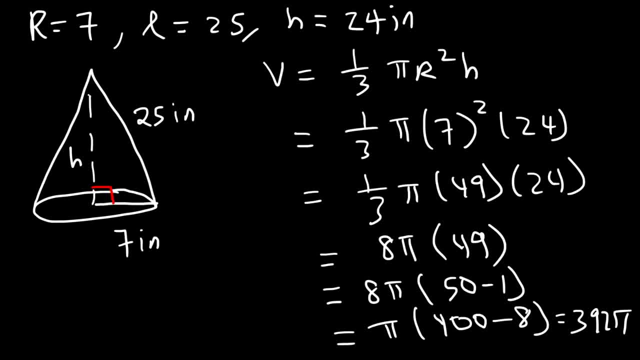 And it turns out that if you type in 8 times 49, it's 392.. So that's going to be the volume. The volume is 392 pi cubic inches. Now let's go ahead and calculate the lateral area And then let's find the surface area. 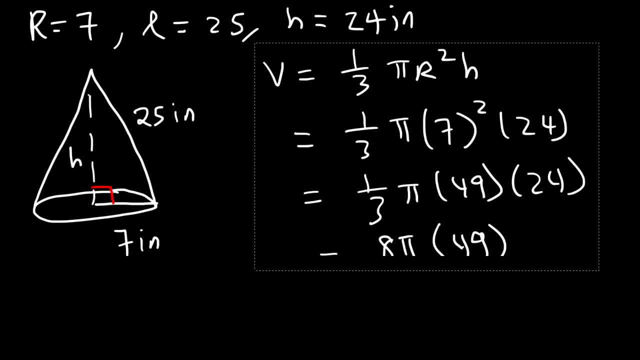 So let's go ahead and calculate the lateral area And then let's find the surface area. So let's start by writing the equation: The lateral area is pi times R times L. So R is 7, L is 25.. Now if you have 7 quarters, that's $1.75. 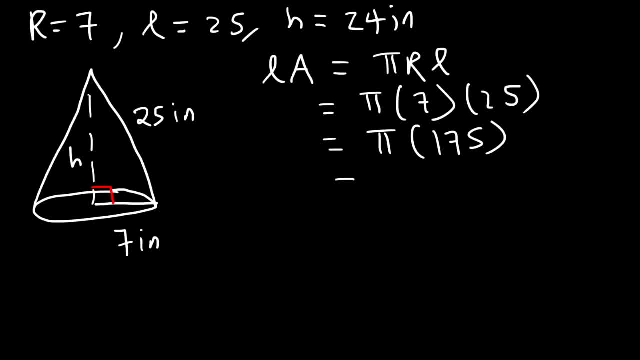 So 7 times 25 is 175.. So the lateral area is 175 pi square inches. Now let's calculate the surface area. So the surface area of the cone is going to be the area of the base plus the lateral area. The area of the base is pi R squared. 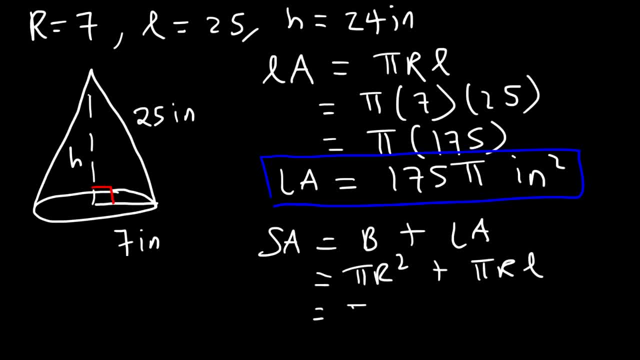 The lateral area is pi R L, So R in this example is 7.. And we know that pi R L, that's 175 pi. Seven squared is 49. So we've got to add 49 pi to 175 pi. 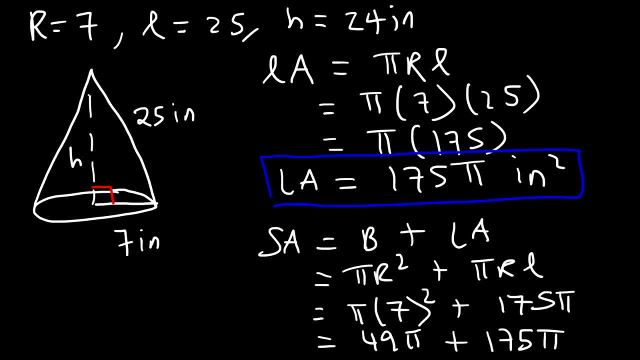 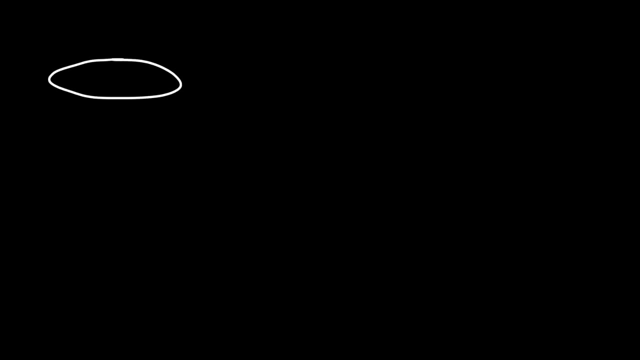 So 179.. I mean, excuse me, 175 pi, That's 224.. So the surface area is 224 pi square inches. And so that's it for this example. Now let's try one more example, for the sake of practice. 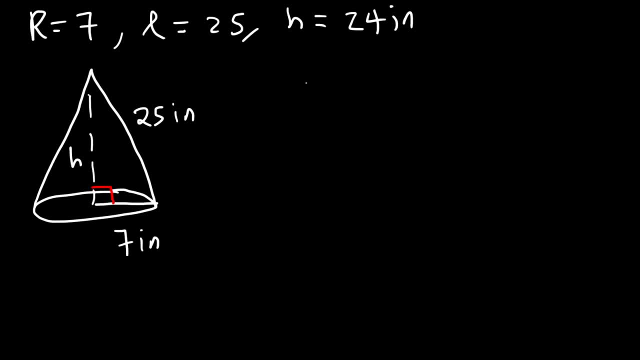 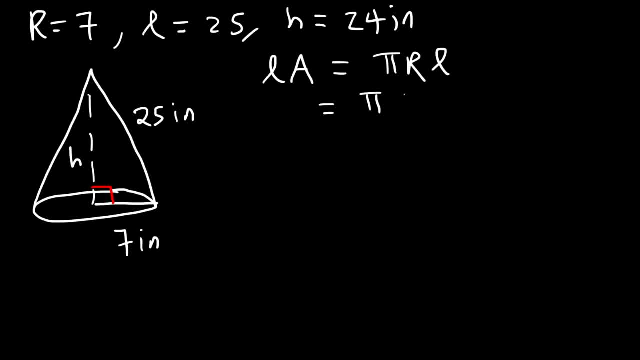 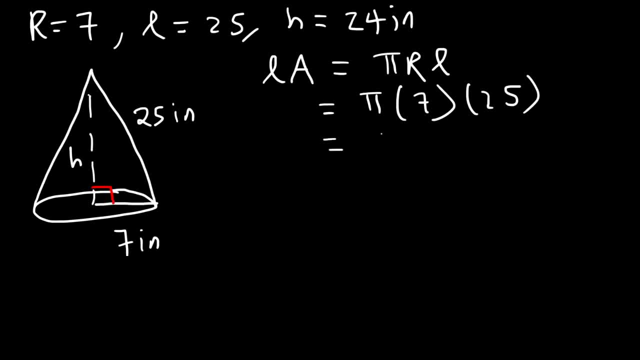 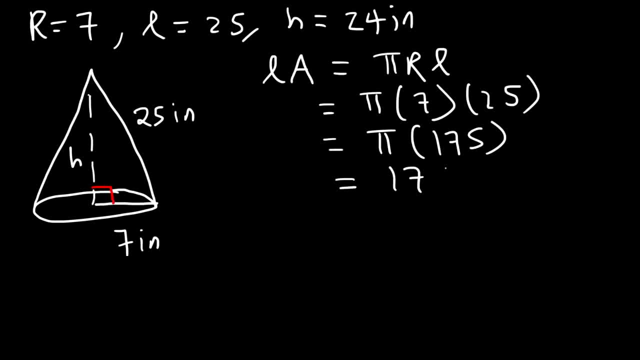 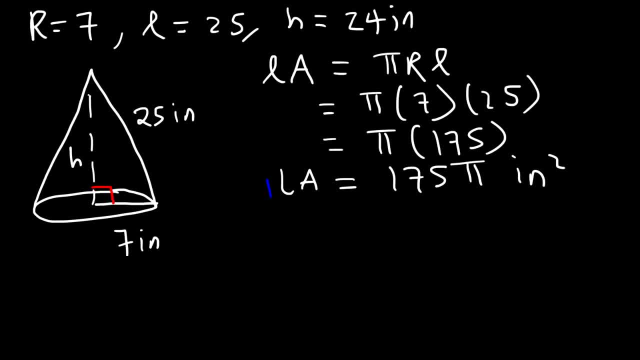 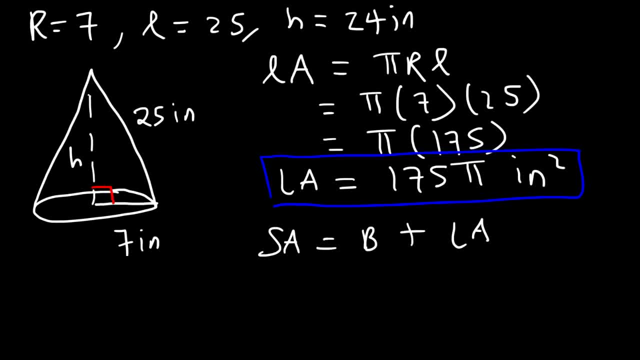 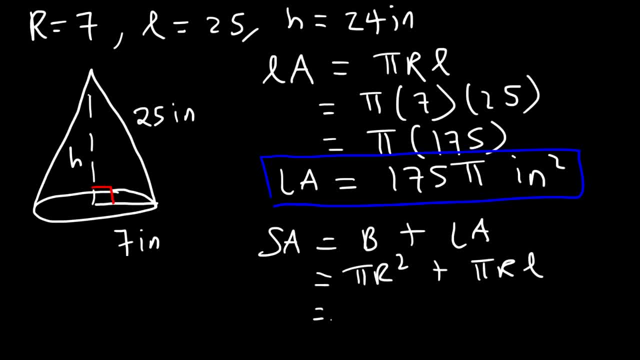 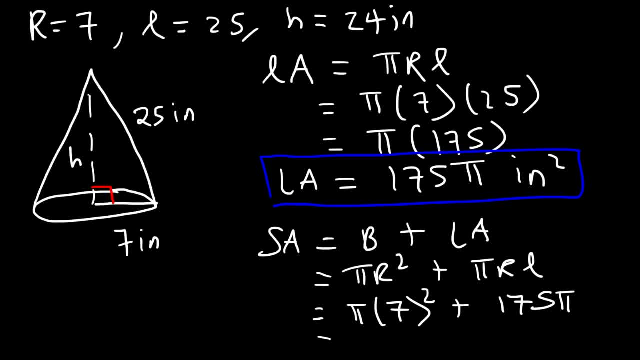 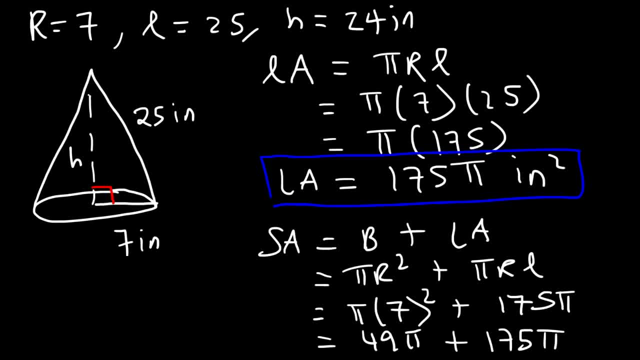 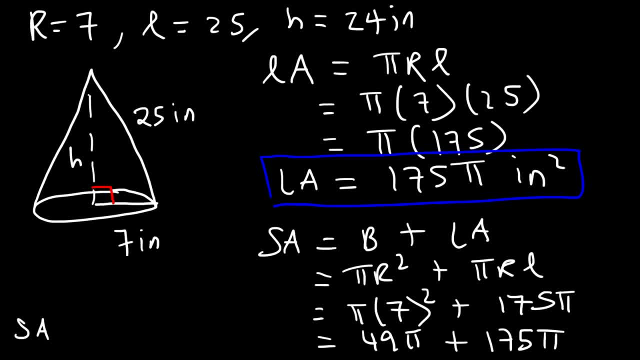 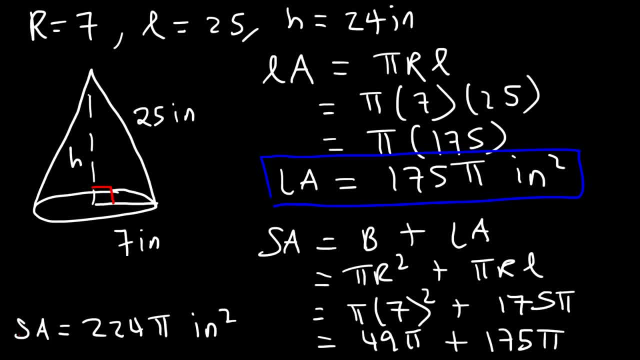 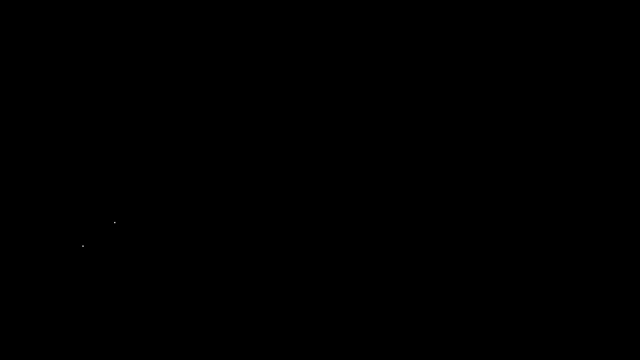 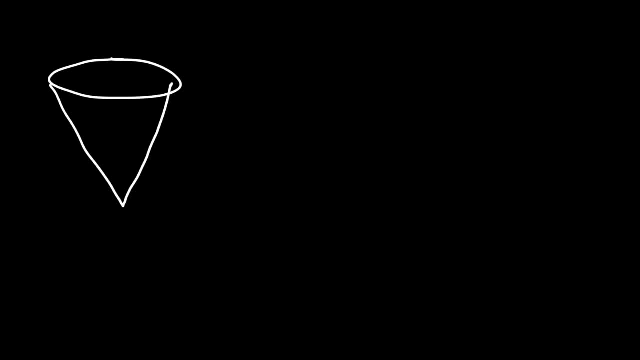 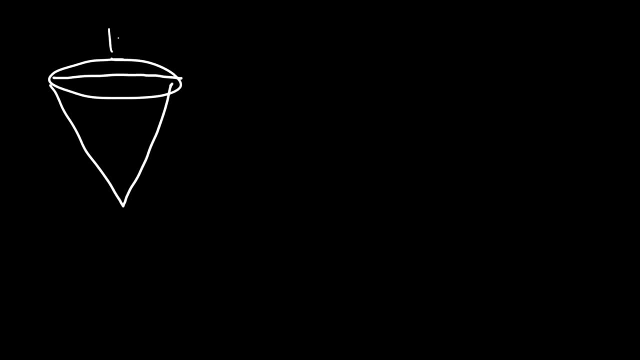 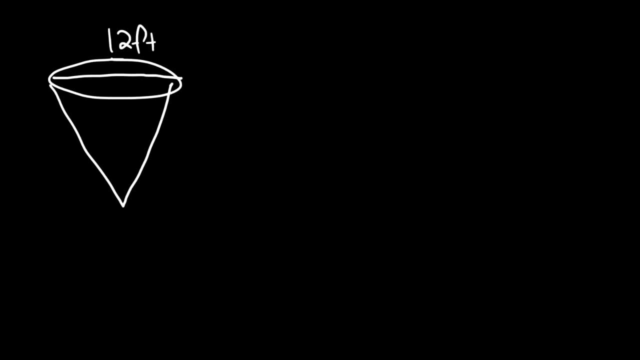 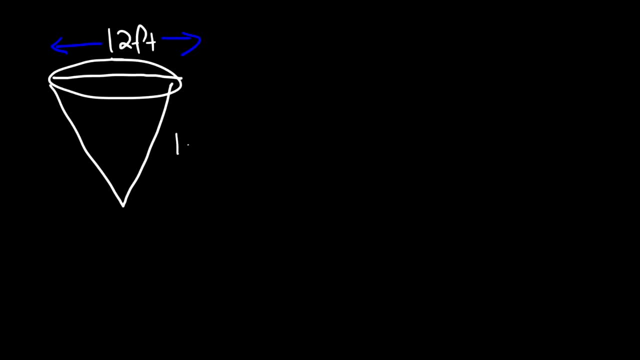 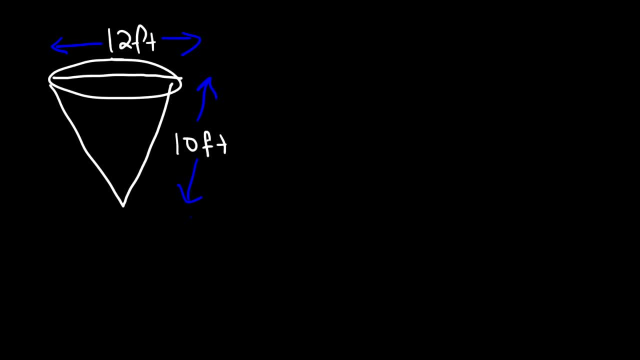 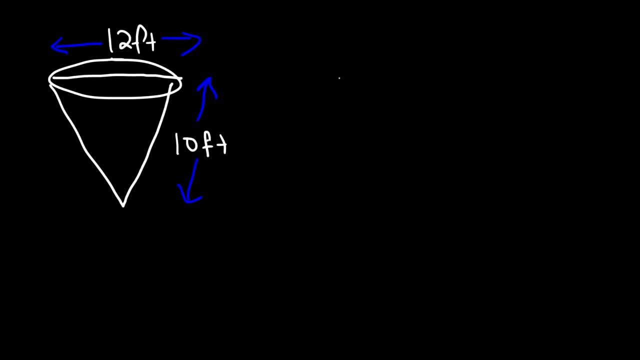 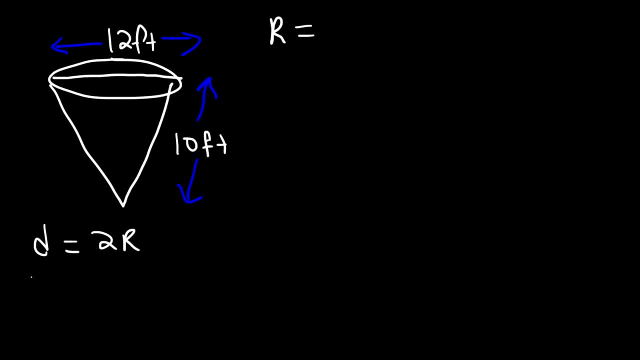 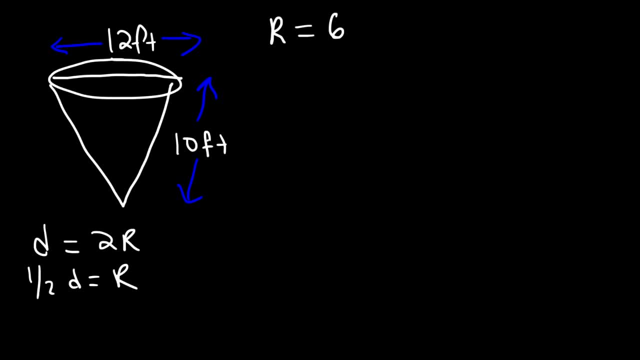 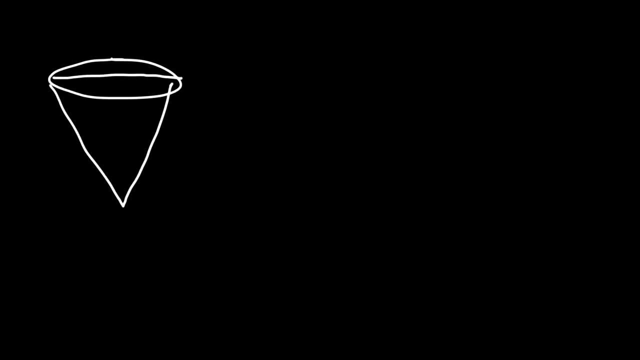 So this time, let's say, if you're given the diameter instead of the radius, Let's say that the diameter is 12 feet And you're given the slant height, which is 10 feet, Go ahead and find the volume, lateral area and surface area. 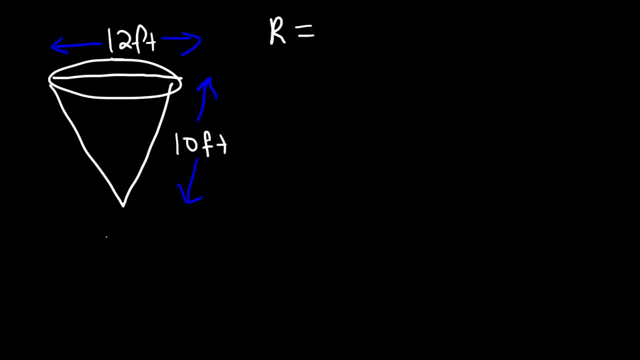 Now the first thing we need to find is the radius. The diameter is twice the value of the radius. so therefore the radius is half of the diameter. So half of 12 is 6, so that's going to give us the radius. 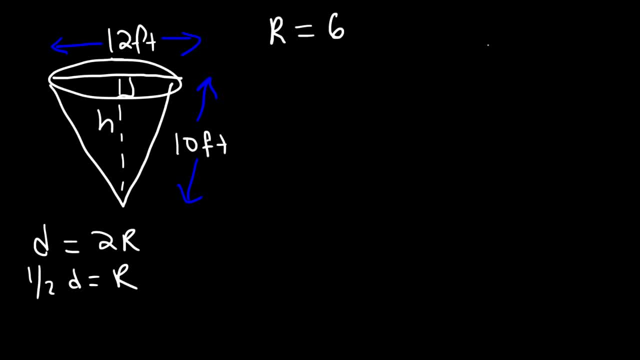 Now we need to find the height. We know that the slant height is 10, but we've got to find the actual height. So, using this equation, L squared is equal to R squared plus H squared. So 10 squared is equal to 6 squared plus H squared. 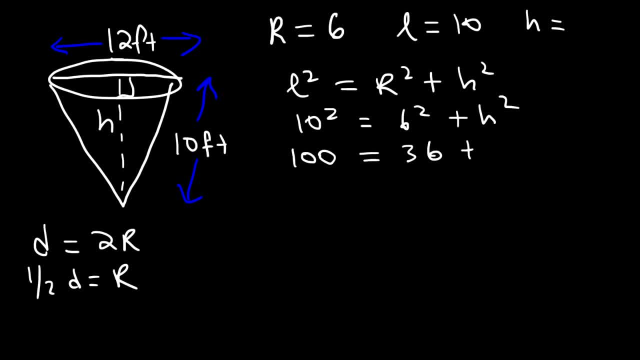 10 squared is 100, 6 squared is 36, and 100 minus 36 is 64.. And the square root of 64 is 8.. So the height of the cone is 8 feet. It's a pretty long cone. 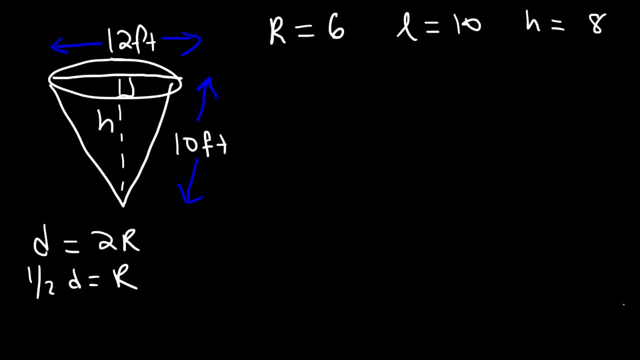 Now let's see, Let's calculate the volume first using this equation: One third pi R squared times the height. So R is 6, H is 8.. 6 squared that's 36.. And if we take 36 and divide it by 3, that's going to give us 12.. 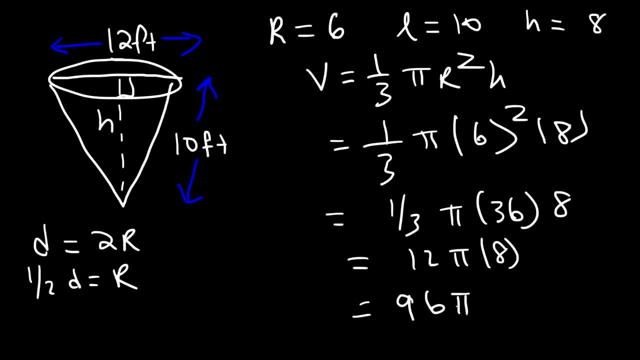 And 12 times 8 is 96. So the volume is 96. It is 96 pi cubic feet. Now that we have the volume, let's go ahead and calculate the lateral area. So that's going to be pi R L. 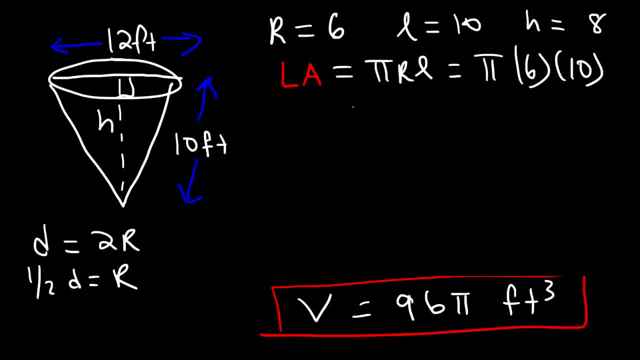 R is 6, L is 10.. 6 times 10 is 60. So the lateral area is 60 pi square feet. Now the last thing we need to do is calculate the surface area. So keep in mind that's going to be the area of the base plus the lateral area. 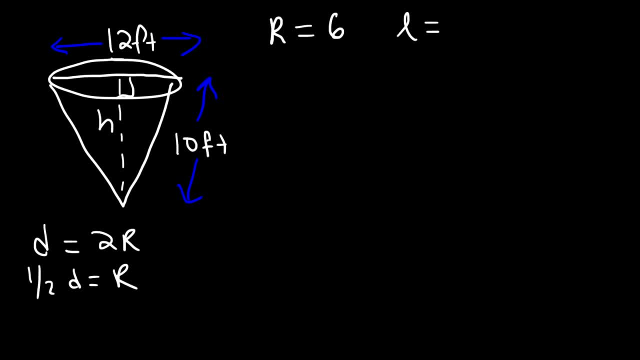 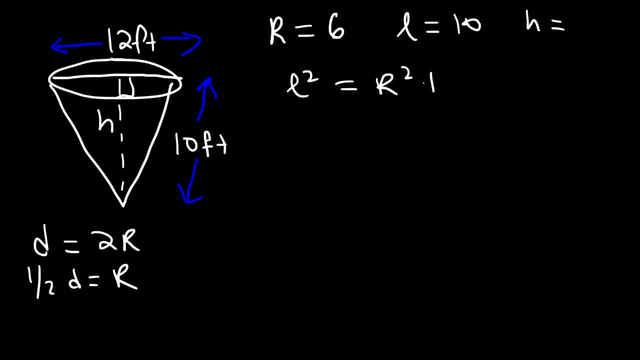 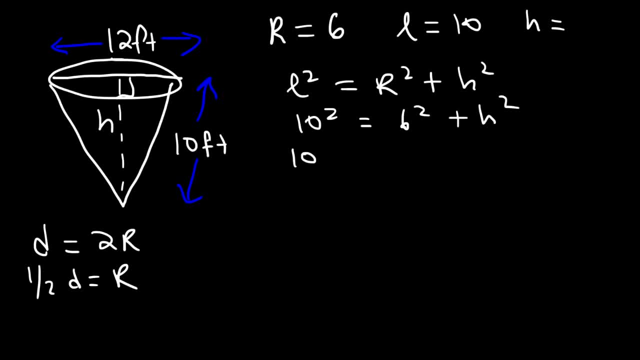 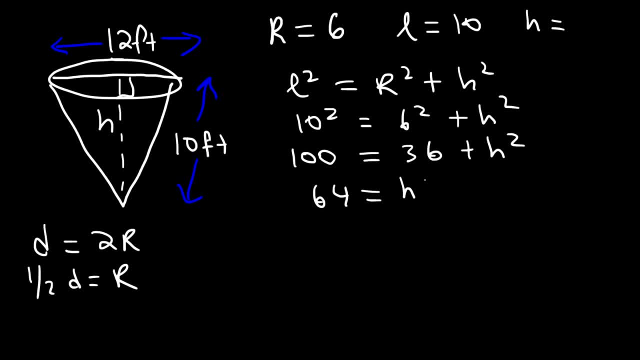 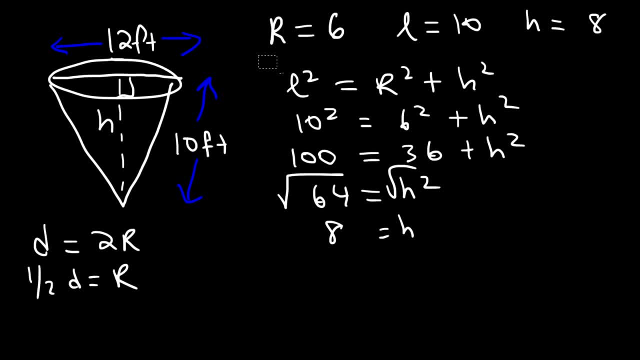 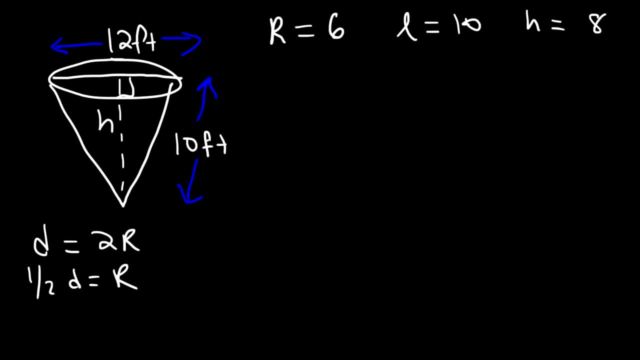 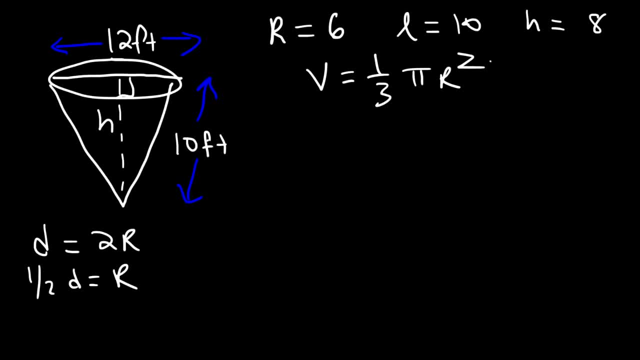 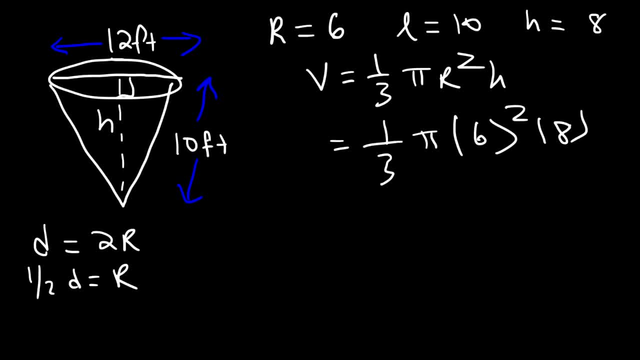 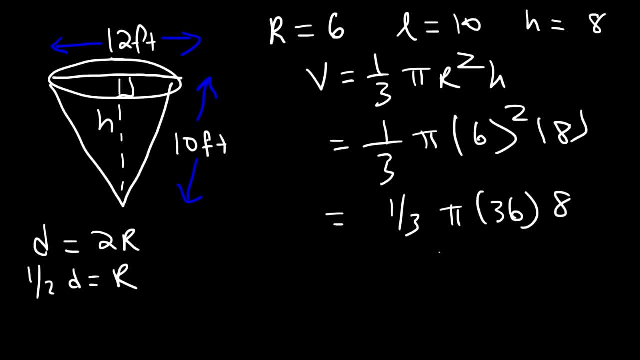 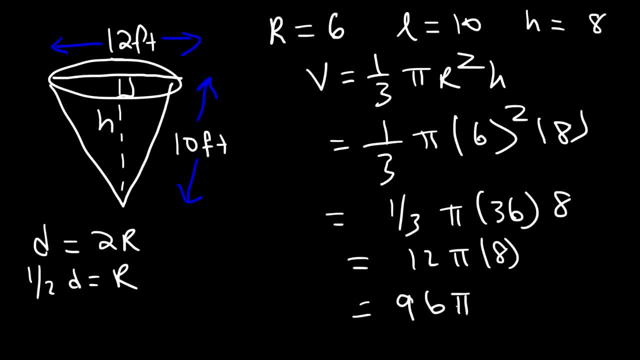 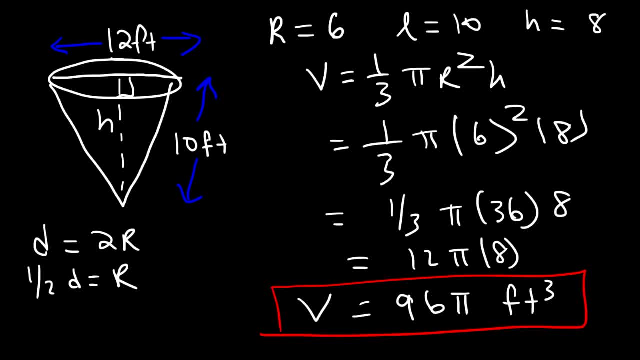 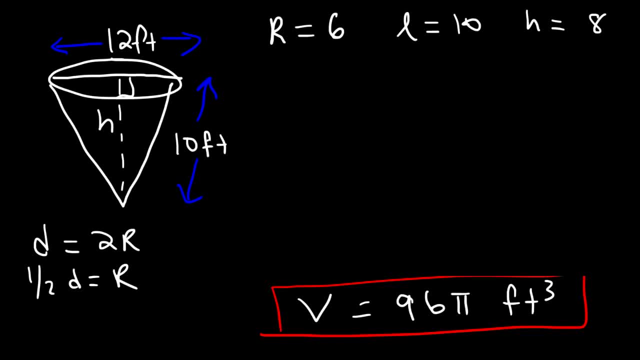 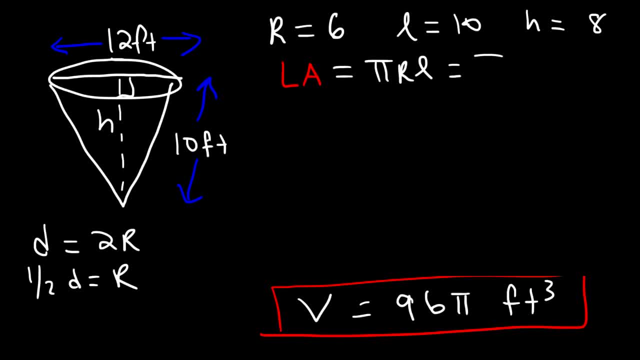 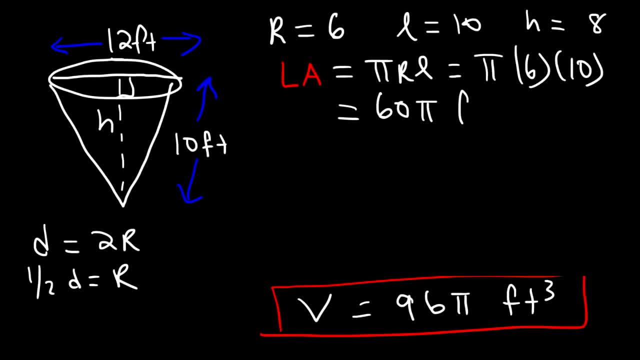 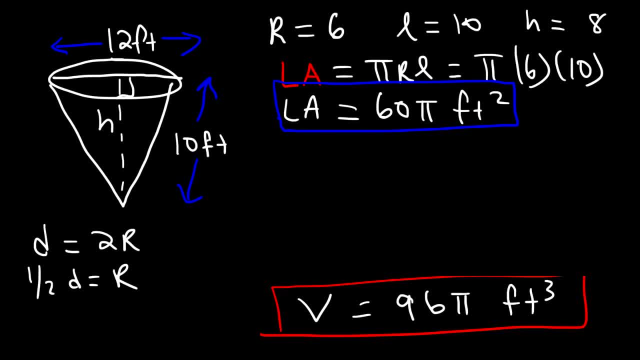 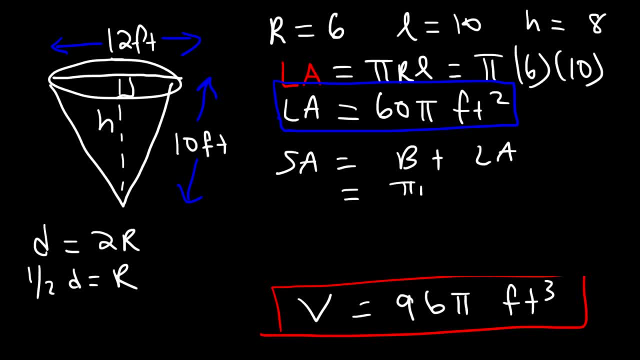 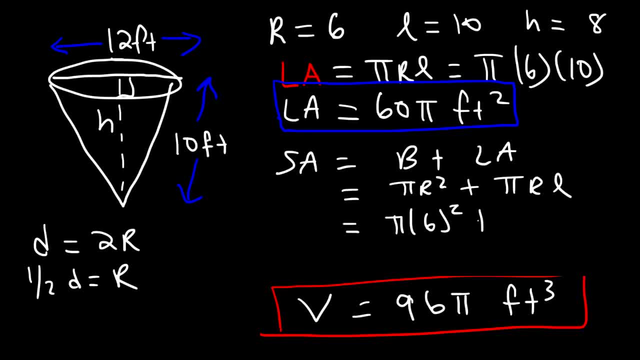 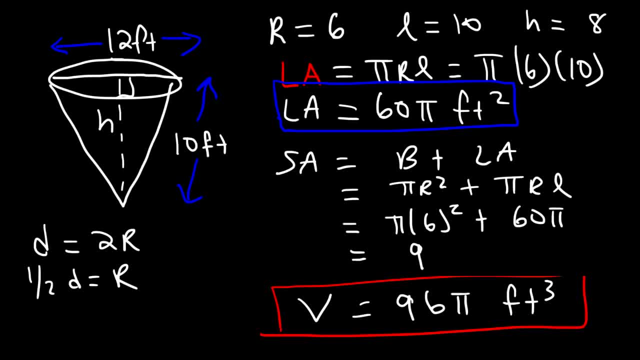 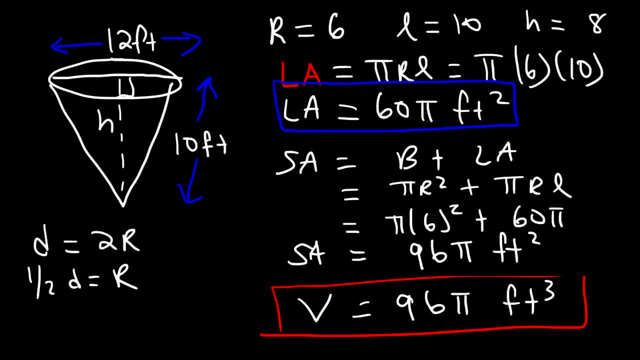 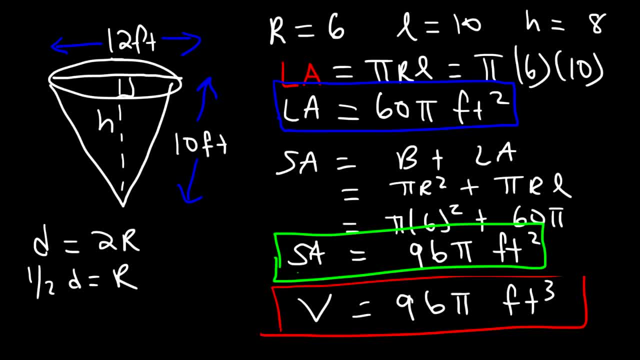 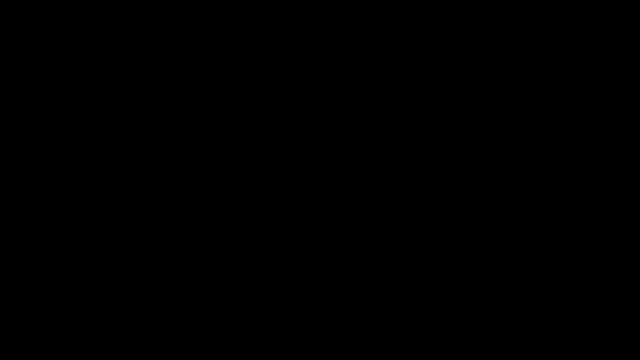 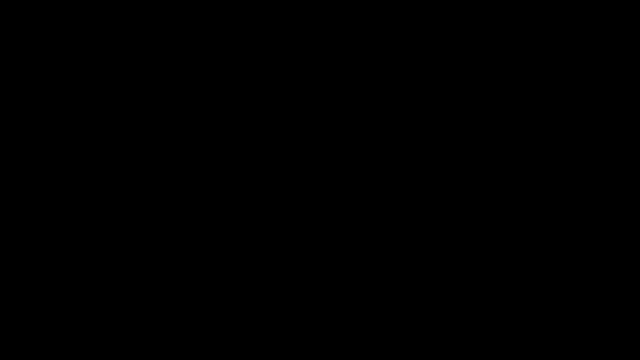 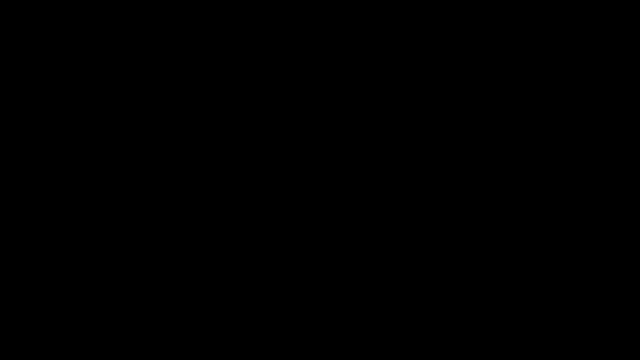 Subtitles by the Amaraorg community. Thank you. 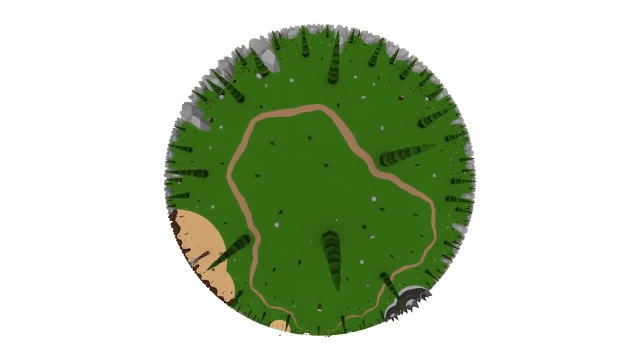 Hyperbolic space is so cool, but if you've ever seen any kind of visualization, odds are it was this or this or, oh god, the worst one. please stop using this one. But none of these really gave me a feeling of what it's like to live in a curved space, and that was the reason I started. 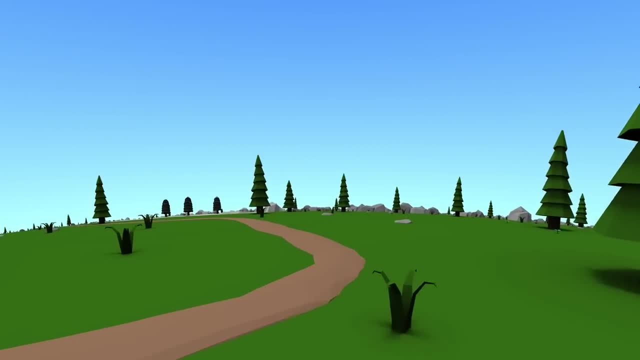 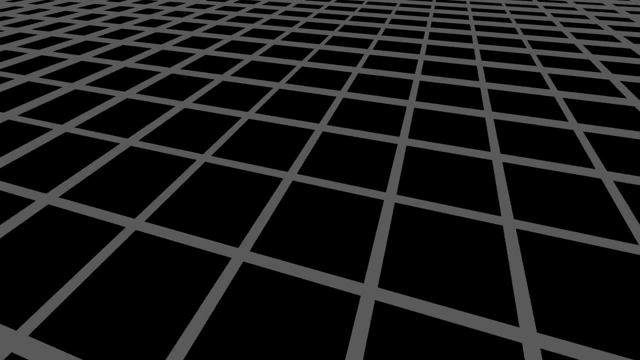 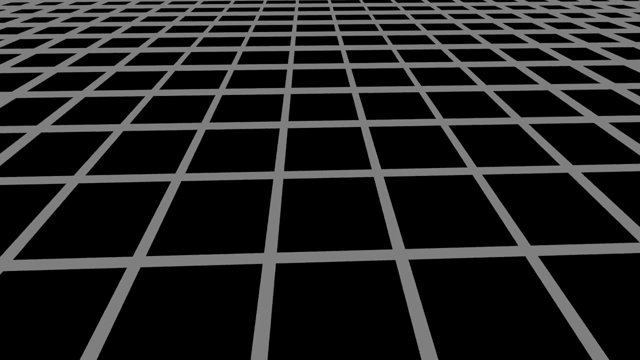 Hyperbolica. So I've come up with what I think is the easiest way to understand hyperbolic space. Let's start off with Euclidean and spherical spaces in two dimensions, and then hyperbolic space in three dimensions come naturally later. So here's just a regular flatland: 2D- Euclidean. 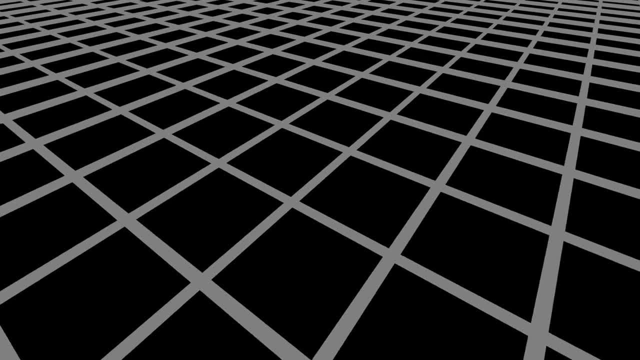 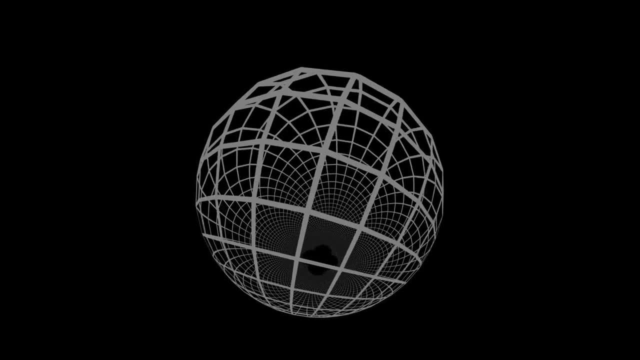 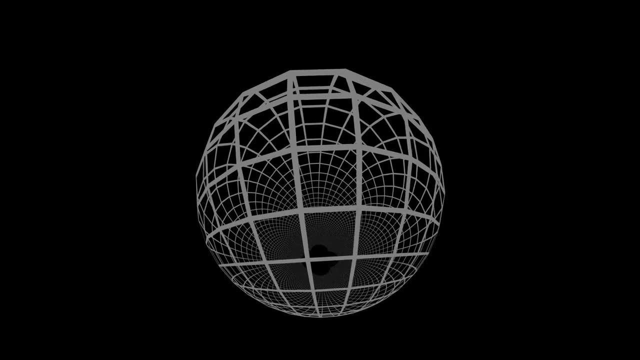 plane. It goes on in every direction and has no curvature. But if we add some positive curvature we get a spherical shell. This is not a solid ball. there's no inside or outside, just an infinitely thin, two-dimensional shell. We're only looking at it in 3D because we are 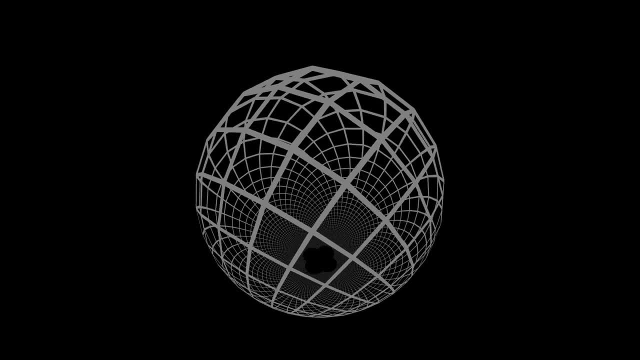 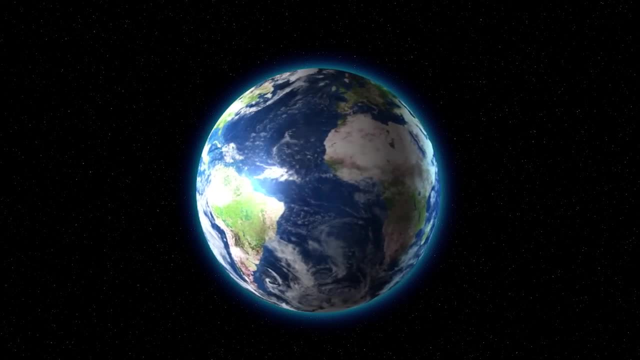 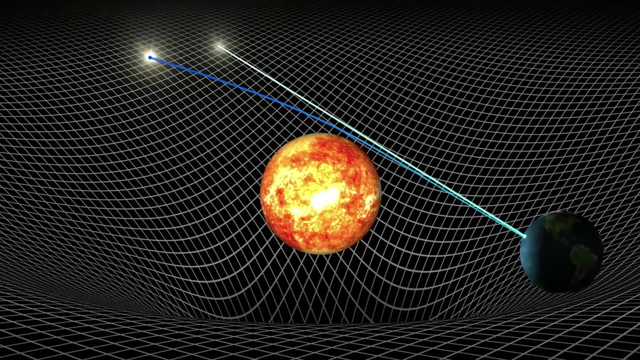 higher dimensional beings. looking down at the flatlanders, You might think this is really similar to us- We're just living on the surface of Earth. But there's actually a big difference, and it has to do with light and lines. Think about light bending around the curved space of a black hole. Light always travels in the shortest path, in a straight line.